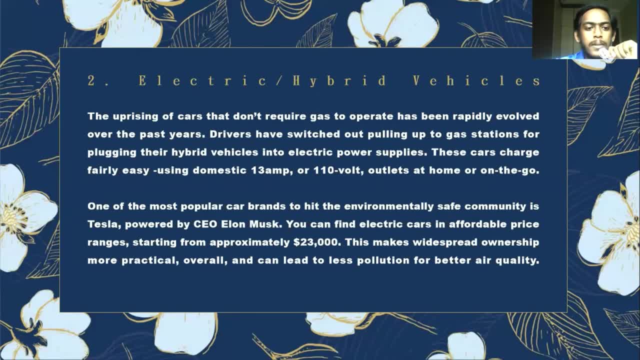 that is eco-friendly, and eco-friendly scooters. Let's move on to the next method, that is, electric or hybrid vehicles. The uprising of cars that don't require gas to operate has been rapidly evolved over the past years. Drivers have switched out cooling up to gas stations for 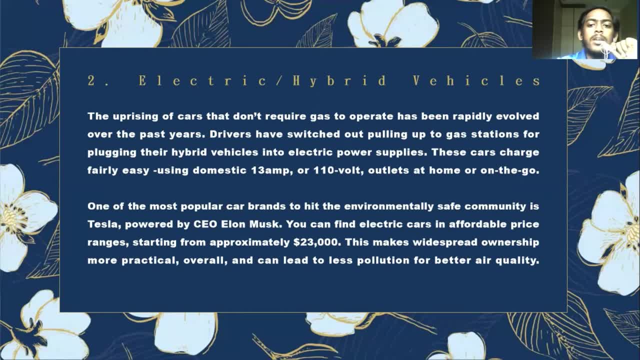 plugging their hybrid vehicles into electric power supplies. These cars charge fairly easy using domestic 13 amp or 110 volt outlets at home or on the go. One of the most popular cars brands to hit the environmentally safe community is Tesla, powered by CEO Elon Musk. 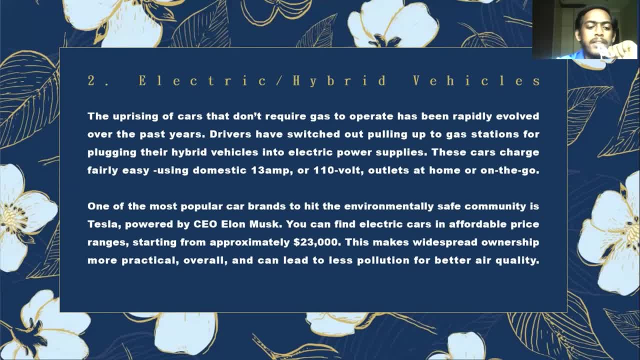 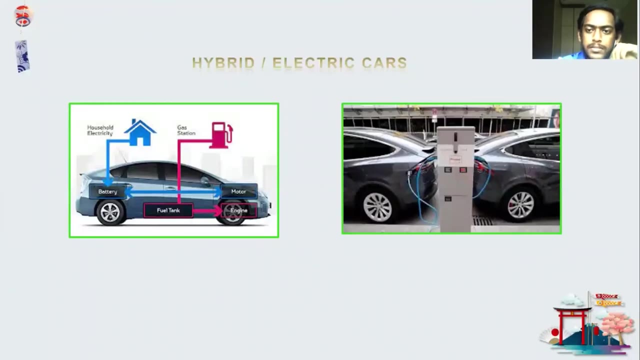 You can find electric cars in affordable price ranges, starting from approximately 23 USD thousand. This makes a widespread opportunity. This makes ownership more practical overall and can lead less population for better air quality. These are the examples of hybrid and electric cars. Nowadays, we can see it in Malaysia too. 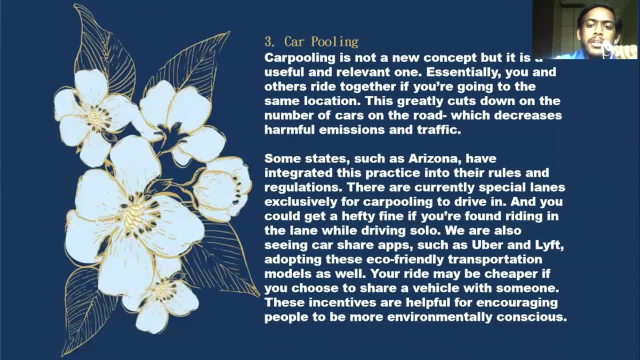 The next. the third method is carpooling. Carpooling is not a new concept, but a useful and relevant one. Essentially, you and other riders together, if you are going to the same location and city, can drive the car more accessible. It is a way to get the full picture in driving. 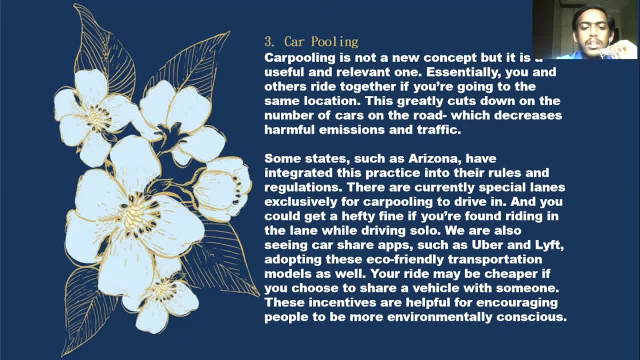 This greatly cuts down on the number of cars on the road, which decreases harmful emissions and gravity. Some states, such as Arizona, have integrated this practice into their rules and regulation. There are currently special lanes exclusively for carpooling to drive in, and you could get it hefty fine if you are found riding in the lane while driving solo. 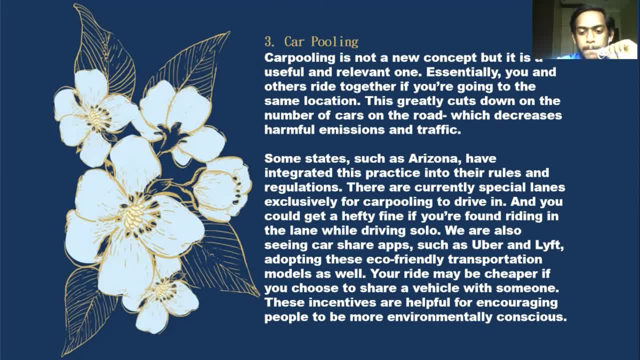 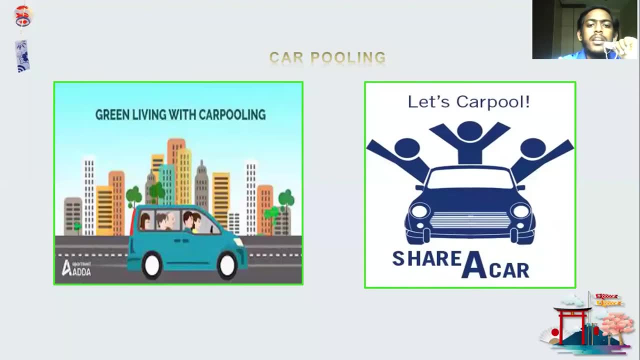 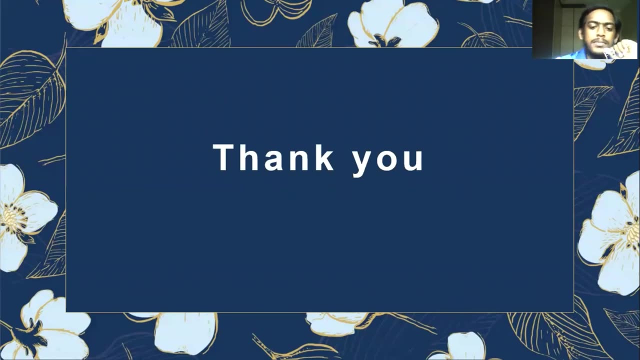 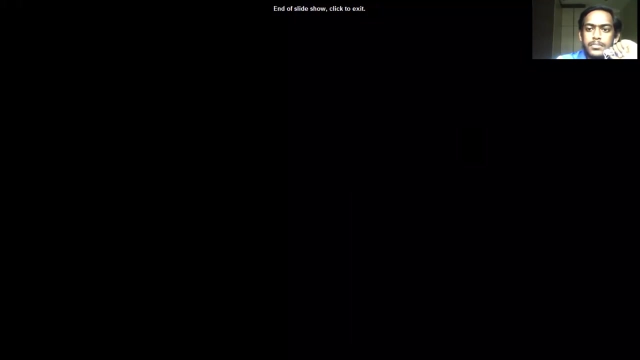 eco-friendly transportation modes models as well. your ride may be cheaper if you choose to share a vehicle with someone. this incentives are helpful and for encouraging people to be more environmentally confused. so these images can explain what is coupling. it's all for my presentation. thank you very much.